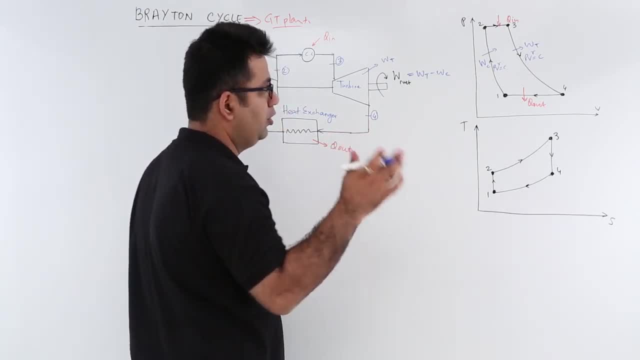 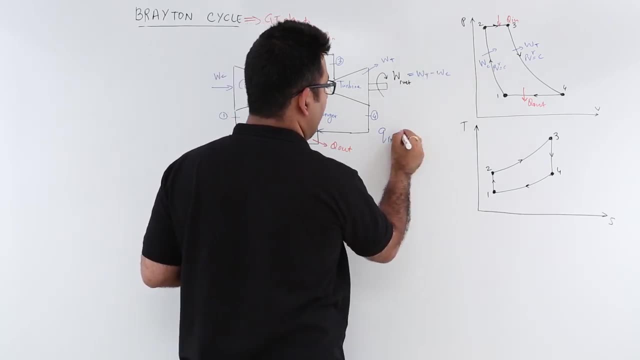 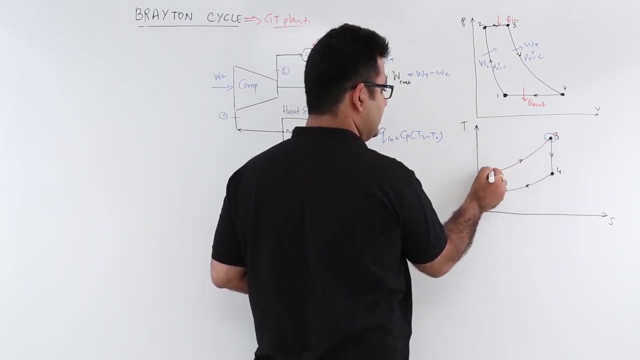 It happens at constant pressure. So if you write down for 1 kg of mass, If you write down Q in, Q, in is 2 to 3.. So you have Cp into T3 minus T2.. You can very well see that T3 is higher as compared to T2.. 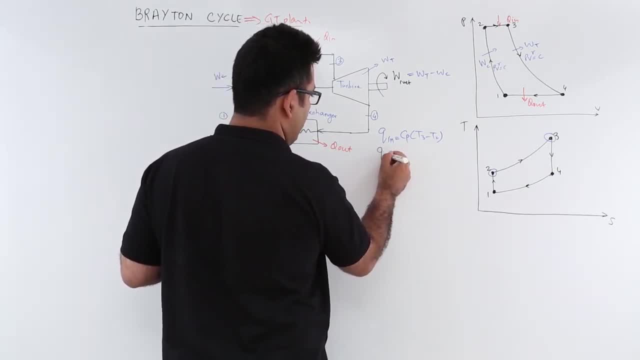 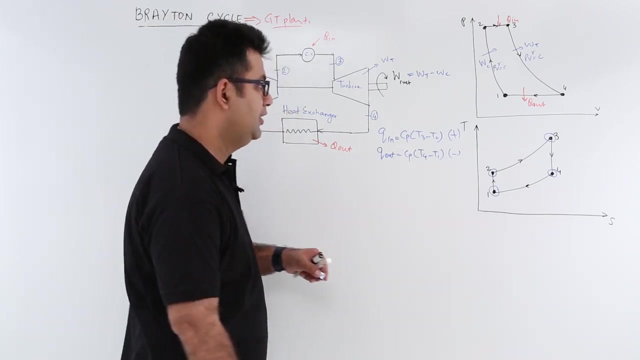 Now, if you find out Q out, That is Cp T4 minus T1.. Now this is taken to be a positive value. This is taken to be a negative value For obvious reasons. Then the network output. First of all, we need to find out the turbine work output. 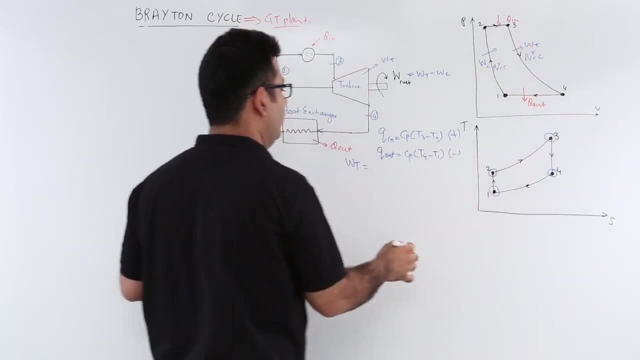 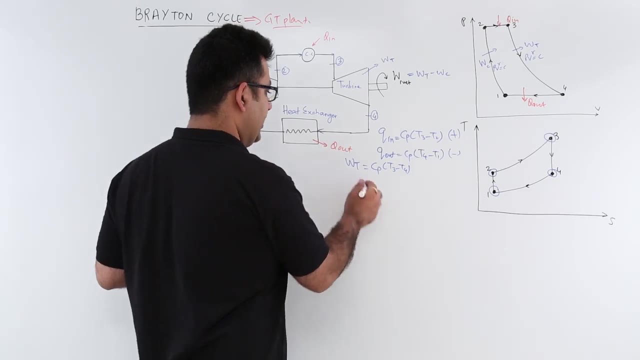 The turbine work output is 3 to 4.. So you will be writing down Cp into T3 minus T4.. Okay, And the network input is from 1 to 2.. So we write down Cp into T2 minus T1.. 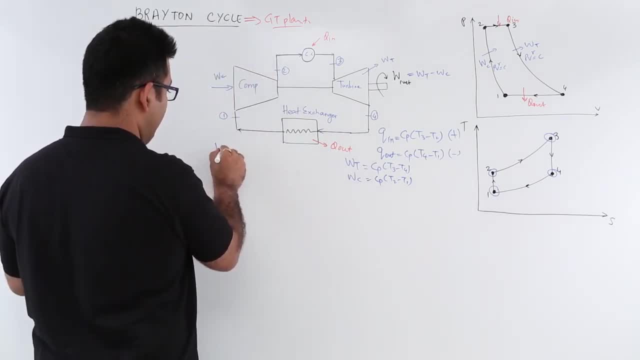 Now the network output. If you write down over here Wnet, This is nothing but Wt minus Wc, And if you divide this by Q in, That would give you the efficiency of the Breton cycle Divided by Q in. 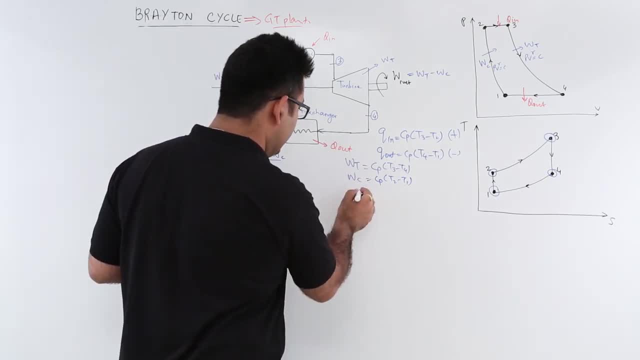 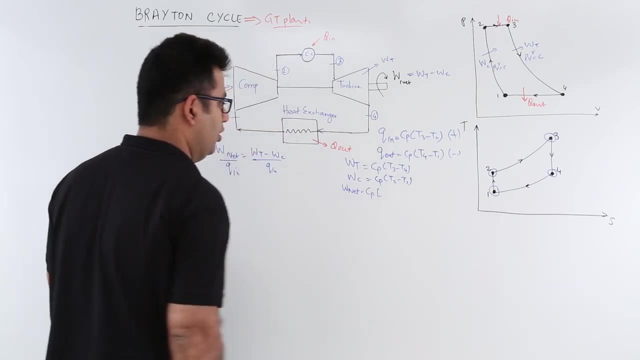 So let's get the values for it. So if you write down this Wnet, You have to subtract these two values So Cp can be taken to be a constant among the two terms. You can have T3 minus T4.. 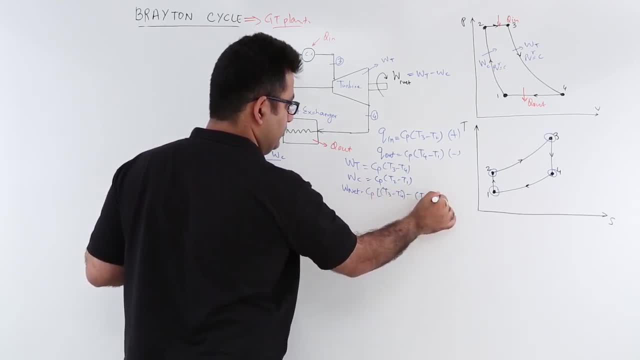 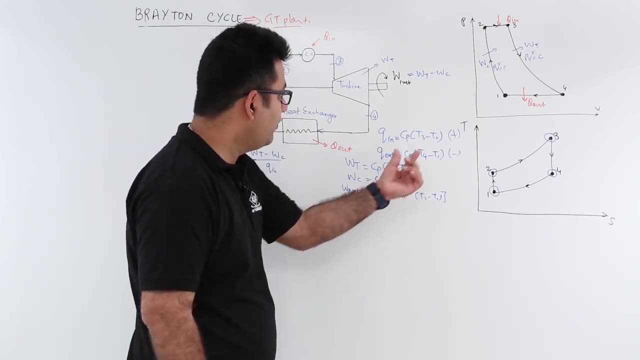 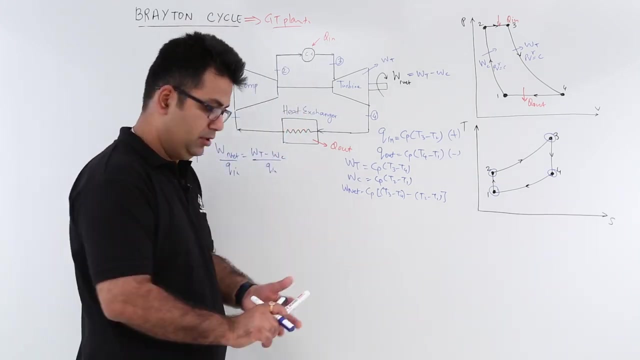 Minus T2 minus T1.. Now look at the expression for Q in. It has a combination of 3 and 2. T3 minus T2.. Let's combine T3 and T2 in the network output equation, So that would become: 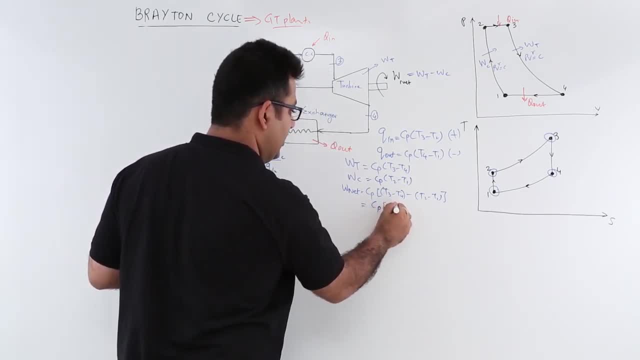 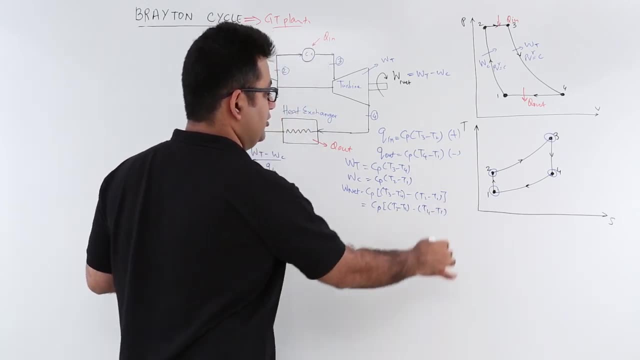 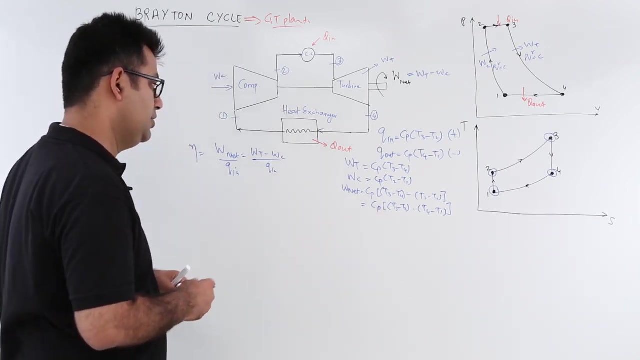 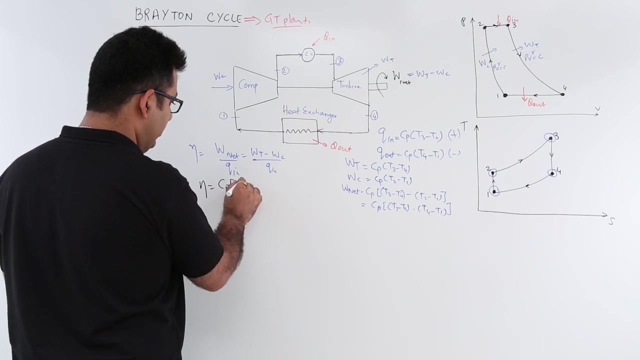 Cp into T3 minus T2.. And then Minus T4 minus T1.. So this is the expression for the network output. Okay, Let's put this into this equation. So The efficiency now becomes Cp Into T3. 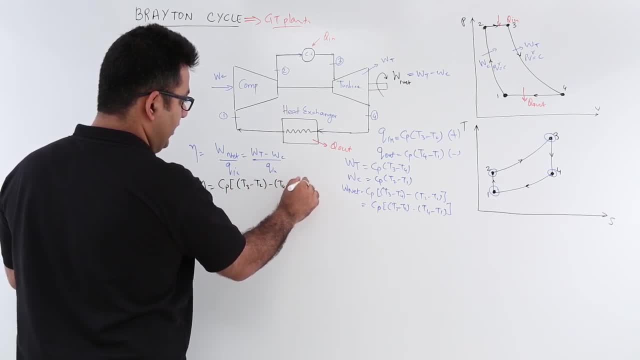 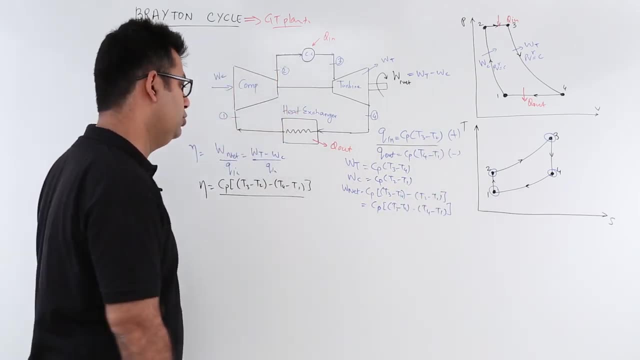 Minus T2.. Minus T4. Minus T1.. Divided by Q, in which is This Cp into T3 minus T2., So you have Cp into T3. Minus T2.. So I can strike off Cp from here. 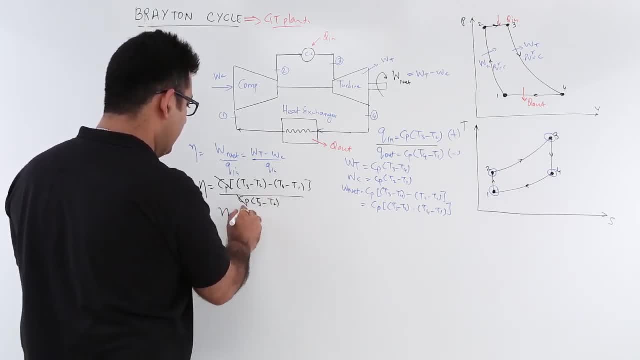 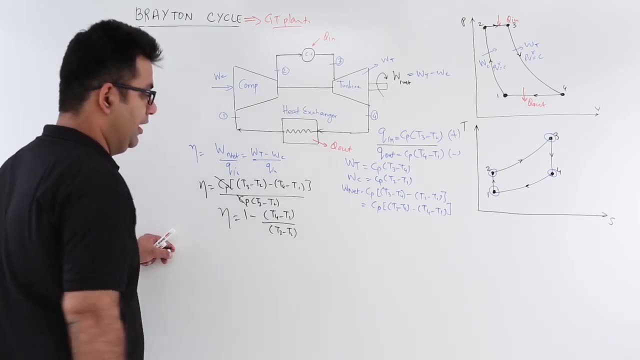 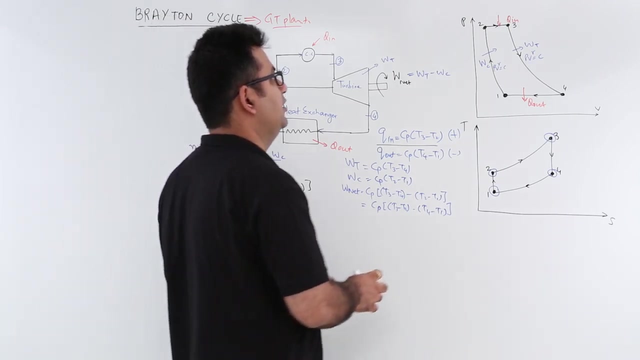 And the Reduced equation will become 1 minus T4, minus T1.. Divided by T3. Minus T2.. Let's Go further in the analysis And look at this pressure, That is P1. To P2.. 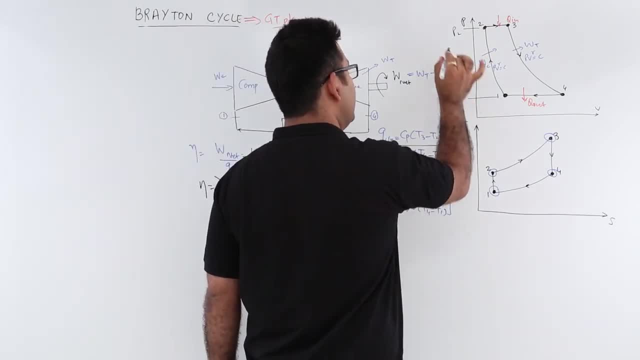 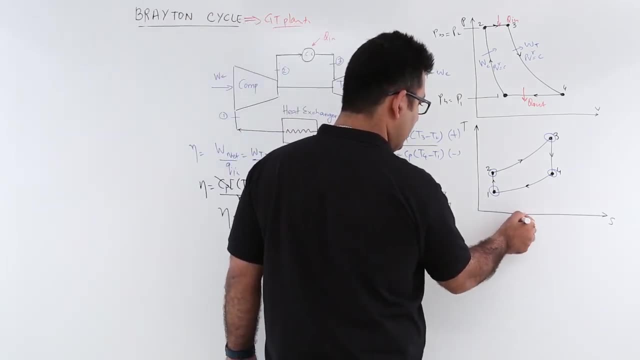 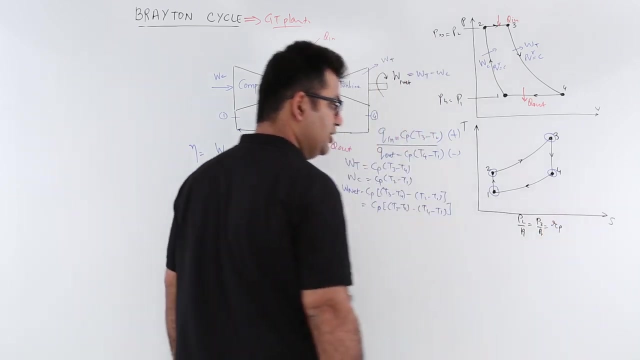 And we know that P1. And P4 are same And P3. And P2 are same. So the ratio P2 by P1. Or P3 by P4. This is the Pressure ratio Rp. So let's get this value. 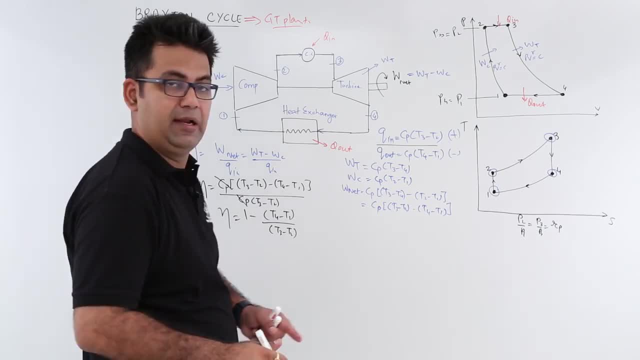 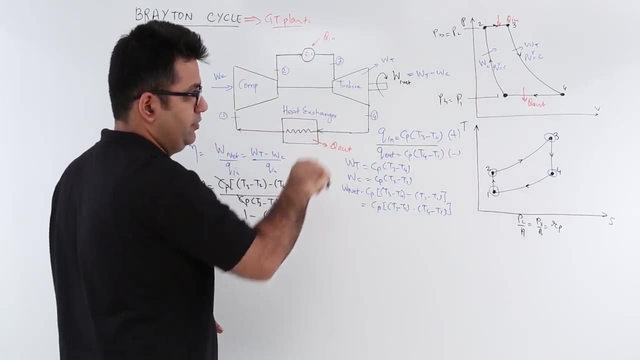 As a function of Rp. Let's do some mathematical Analysis for that. So let's take two processes. Let's take the two isentropic processes, So let's take the first one as 1,2.. So for 1,2.. 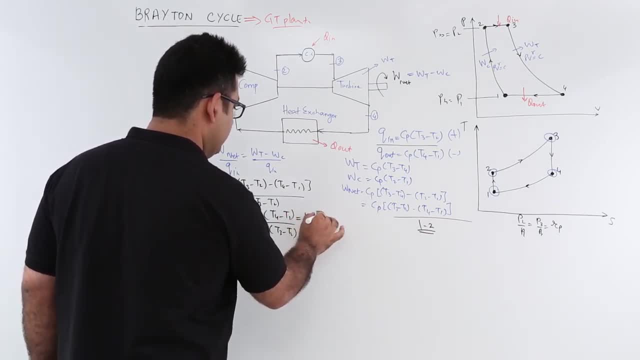 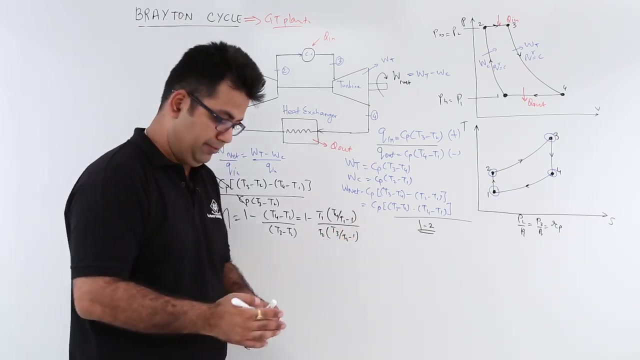 Before I do that, T1 common from here You get T4 by T1. Minus 1. By And T2 common from the bottom: T3 by T2. Minus 1.. Ok, So Now 1,2.. 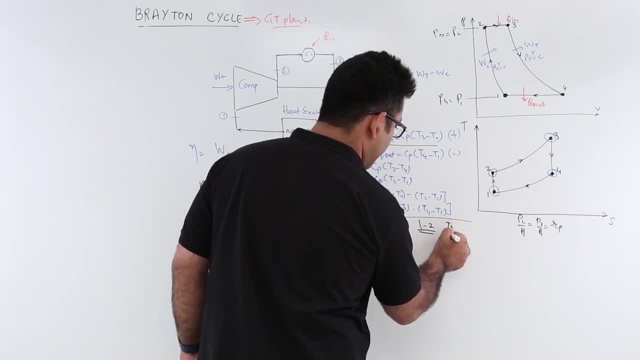 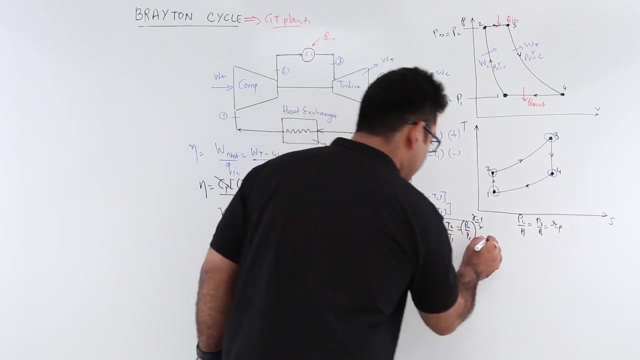 If you write down 1,2.. T2 by T1. That's the temperature ratio Between the two states. This is equal to P2.. By P1. To the power: gamma minus 1.. By gamma, Now, P2 by P1 is the pressure ratio. 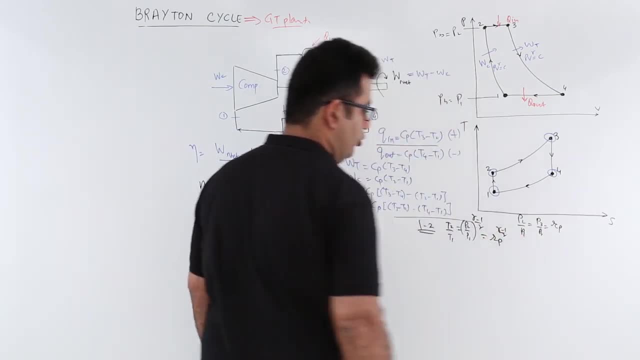 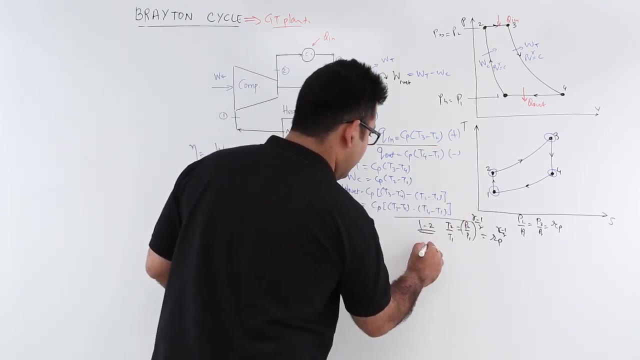 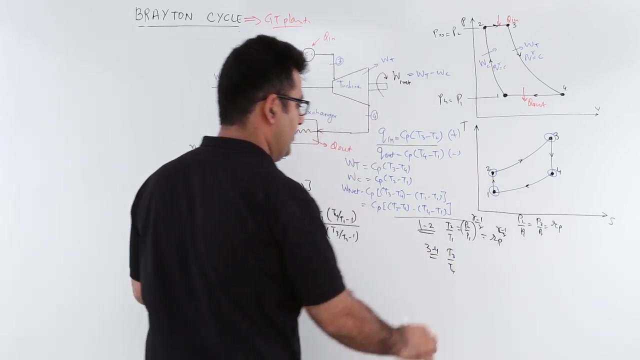 So this becomes equal to Rp, To the power gamma minus 1 by gamma. Ok, And For process: 3,4.. If I write down again 3,4.. For 3,4. I can write down T3.. 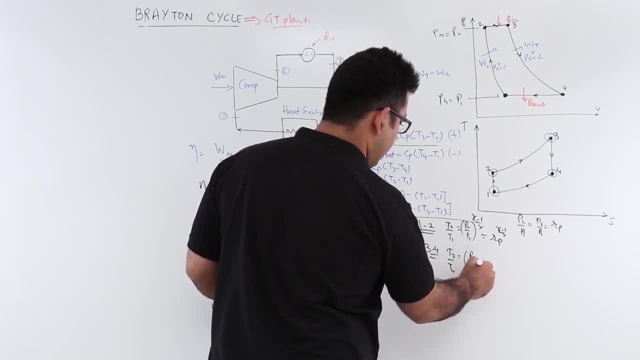 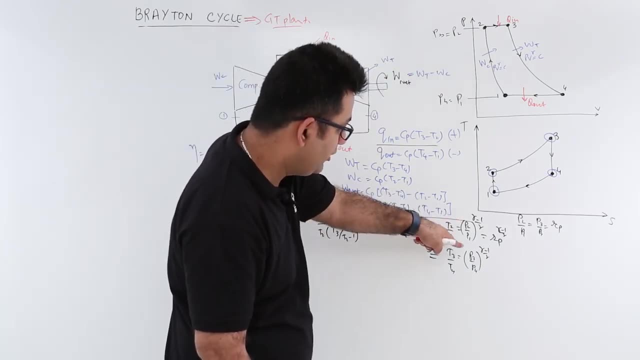 By T4. Is equal to T3 by T4.. To the power: gamma minus 1 by gamma. Now you can see here That P2 and P3 are same. So this P2 is equal to this P3.. 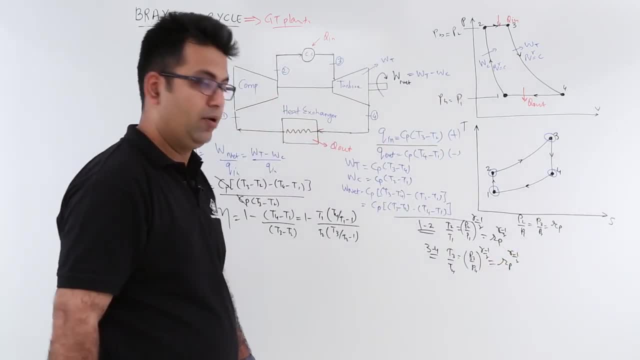 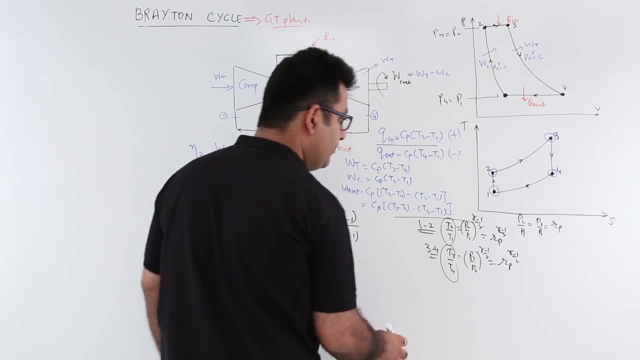 And P1 and P4 are same, So this again becomes Rp to the power gamma minus 1 by gamma. Ok, Now means T2 by T1 is equal to T3 by T4. So let's write this down. 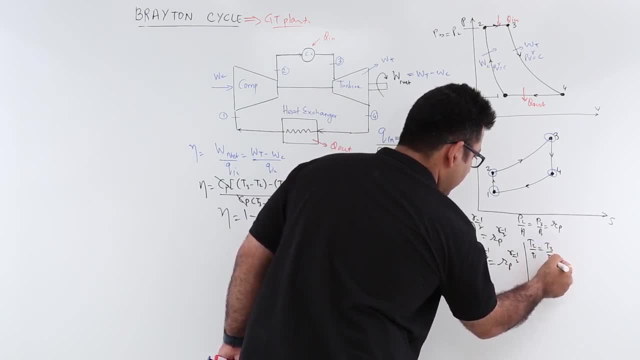 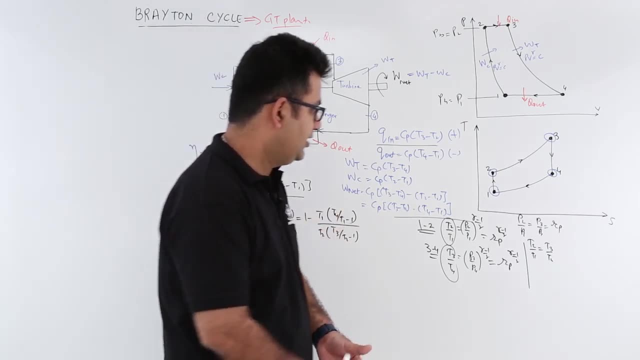 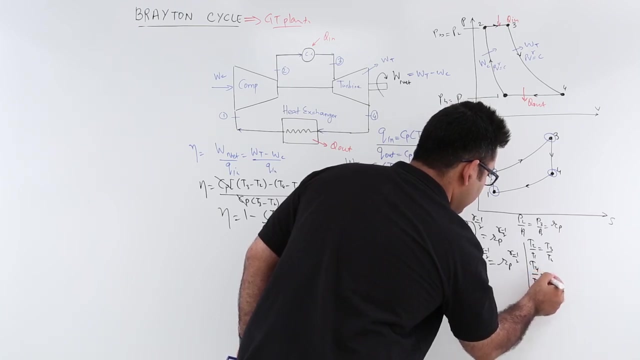 So you have: T4 by T1. Is equal to T3 by T4. So now you need to cancel off T4 by T1. And T3 by T2. So let's swap these. So bring T2 down and take T4 up there. 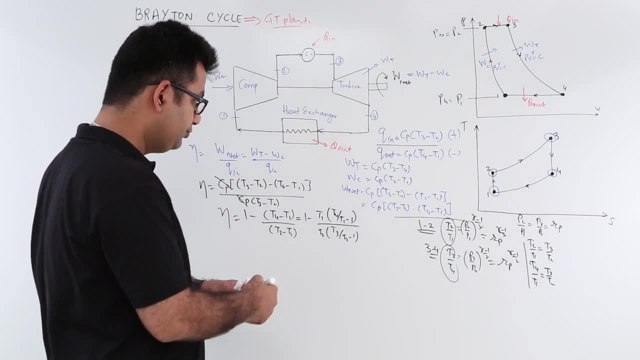 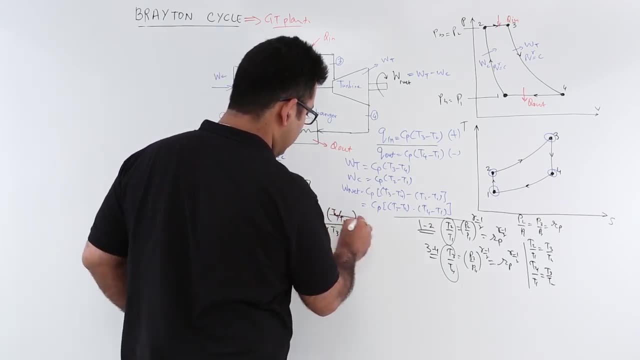 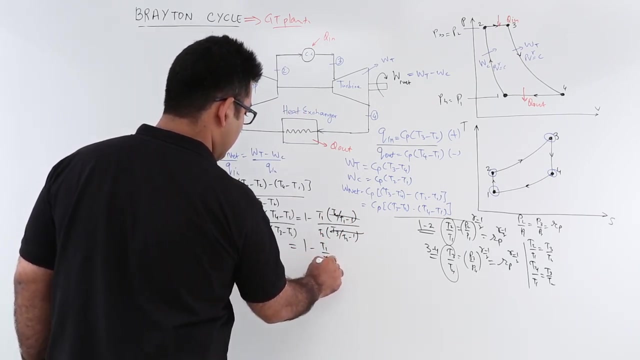 You have: T4 by T1. Is equal to T3 by T2.. So this T4 by T1. Is equal to T3 by T2.. Ok, So you are just left with 1 minus T1 by T2.. 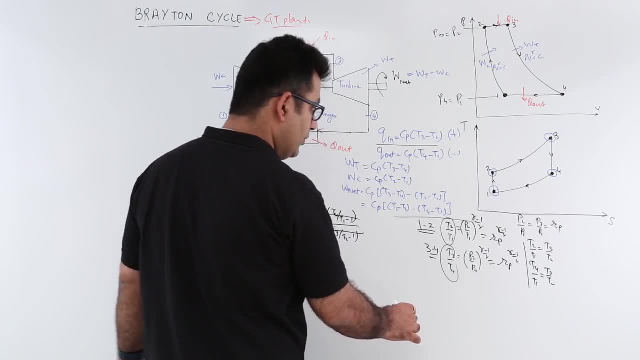 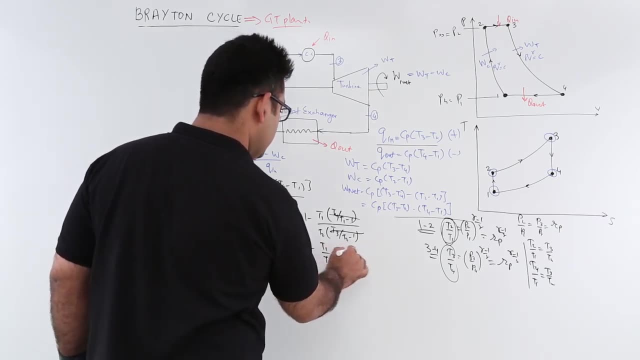 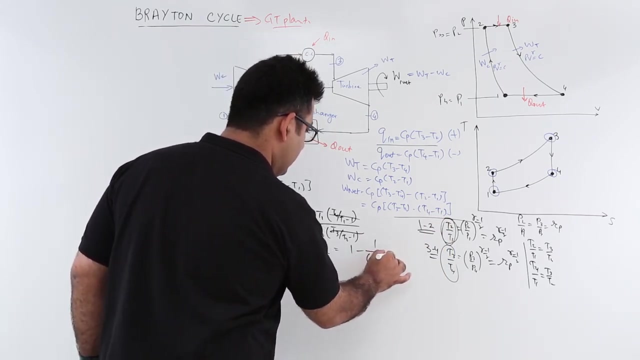 Ok Now T1 by T2. If you look at T2 by T1. This is Rp to the power gamma minus 1 by gamma. So this becomes 1 minus 1 by Rp to the power Gamma minus 1 by gamma. 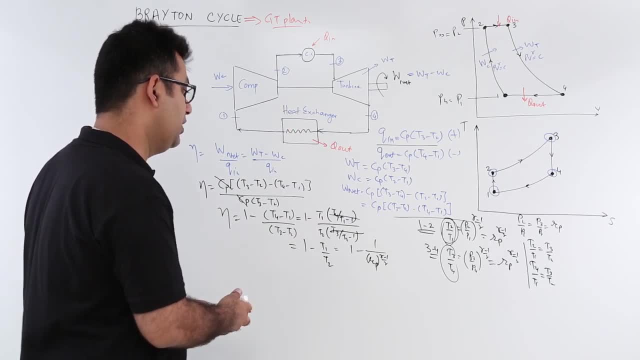 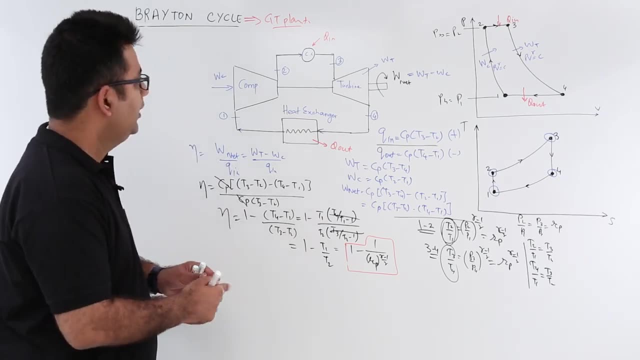 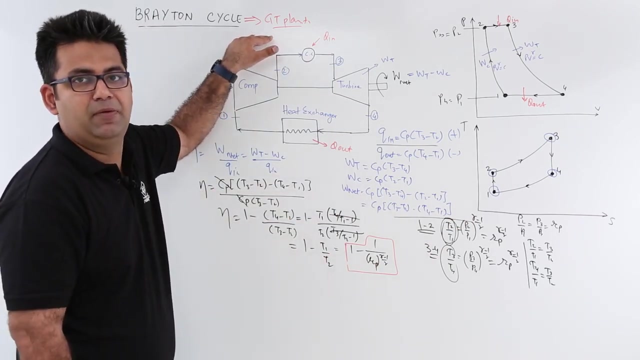 So this Is the expression For the Efficiency of The Brayton cycle. So I hope you understood this Entire mathematical analysis For Brayton cycle, which is The cycle for the gas turbine plants. These are the essential Components.